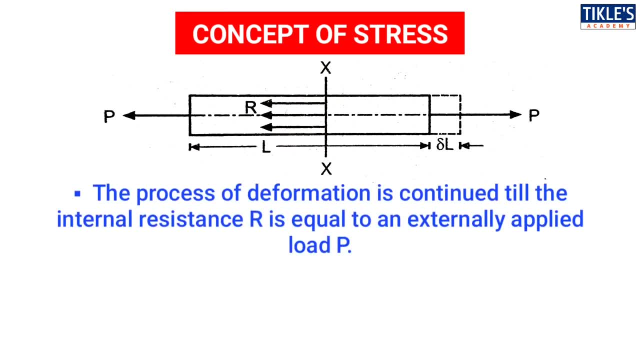 XX. The process of deformation is continued till the internal resistance R is equal to an externally applied load P. If the internal force R is unable to resist this deformation fully, the deformation continues Till the failure takes place. the internal resistive force to deformation per unit cross-sectional. 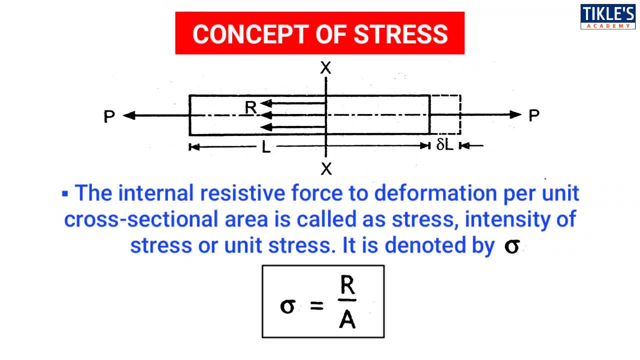 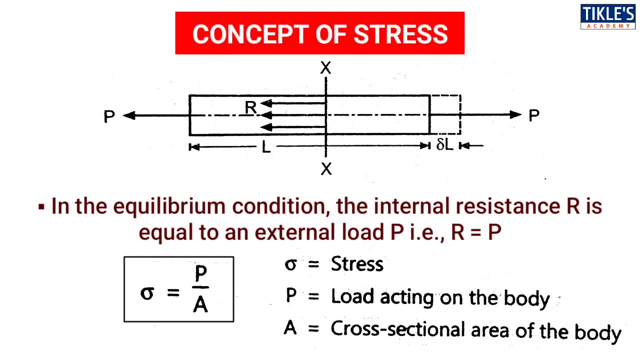 area is called as stress, intensity of stress or unit stress. It is denoted by sigma and given by. sigma equals to R by A. In the equilibrium condition, the internal resistance, R, is equal to an external load, P, ie R equals to P. Therefore, sigma equals to P by A, where sigma 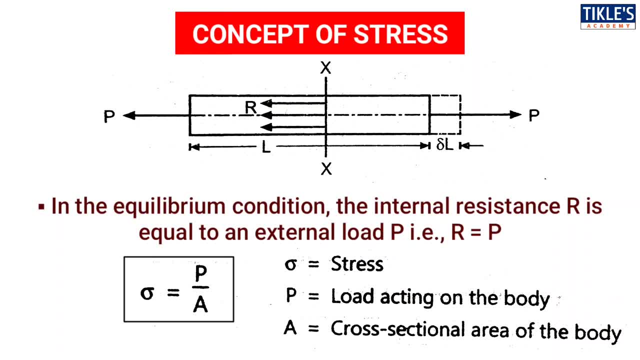 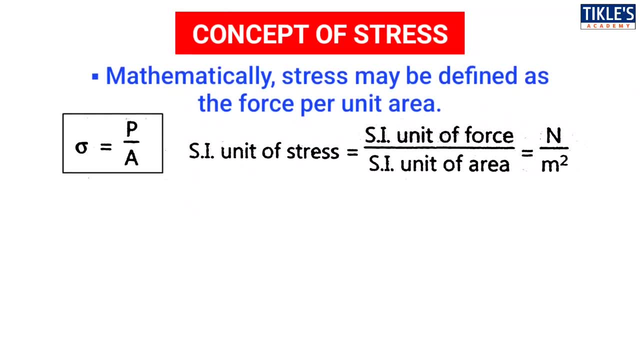 is the stress, P is the load acting on the body, A is the cross-sectional area of the body. Mathematically, stress may be defined as the force per unit area. Now let us see the SI unit. SI unit of stress equals to SI unit of force divided by SI unit. 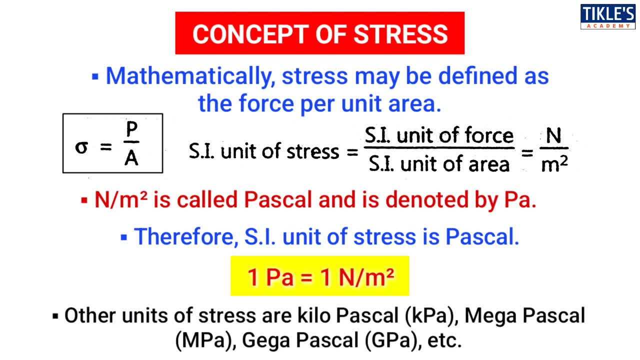 of area which equals to Newton N divided by m square. ie m square. So Newton per m square is called Pascal. SI unit of stress is called Pascal and is denoted by Pa. Therefore SI unit of stress is Pascal. 1 Pascal equals to 1 Newton per m square. Other units of stress are Kilo Pascal. 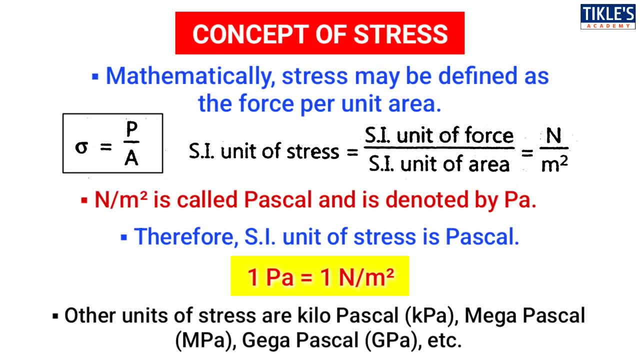 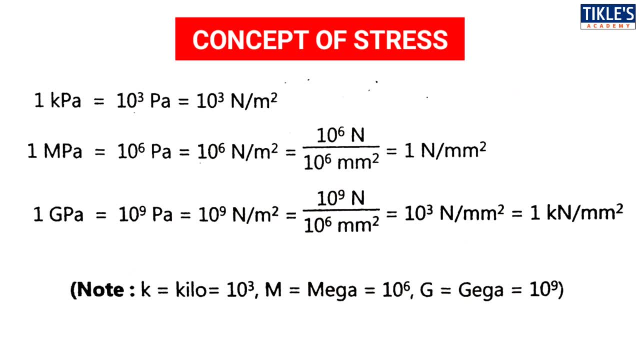 ie KPa, Mega Pascal ie MPa, Giga Pascal, ie GPa, etc. 1 Kilo Pascal equals to 10 to the power 3 Pascal, or 10 to the power 3 Newton per m square, 1 Mega Pascal equals. 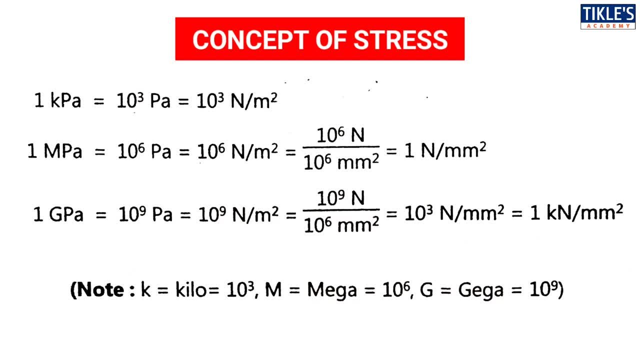 to 10 to the power 6 Pascal, or 10 to the power 6 Newton per m square, or 10 to the power 6 Newton per 10 to the power 6 mm square, or 1 Newton per mm square, and 1 Giga Pascal equals. 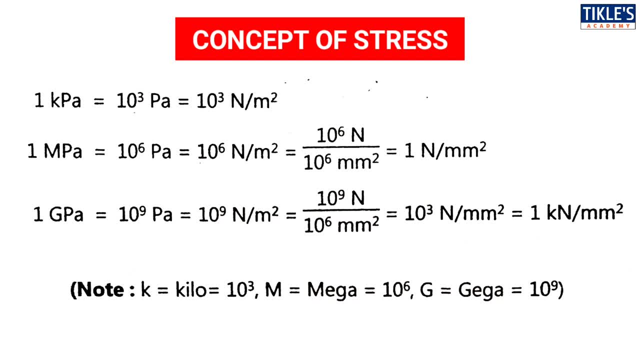 to 10 to the power 9 Pascal, or 10 to the power 9 Newton per m square, or 10 to the power 9 Newton by 10 to the power 6 mm square, or 10 to the power 3 Newton per m square, or 10 to. 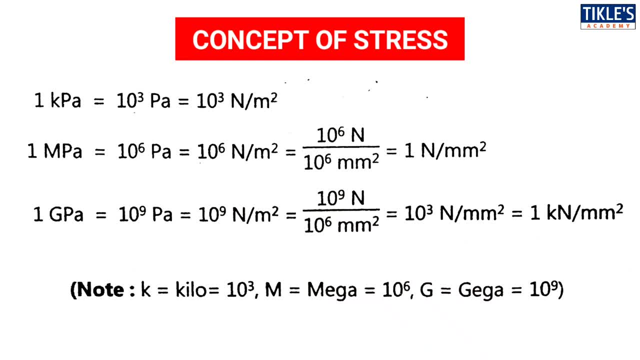 the power: 3 Newton per m square or 10 to the power: 9 Newton by 10 to the power: 6 mm square Newton per mm square or 1 kilo Newton per mm square. Here K stands for kilo, it means 10 to. 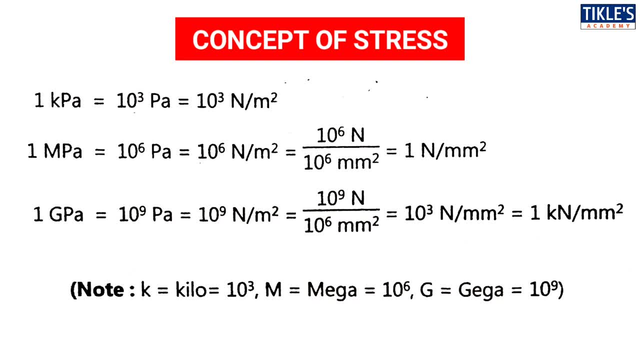 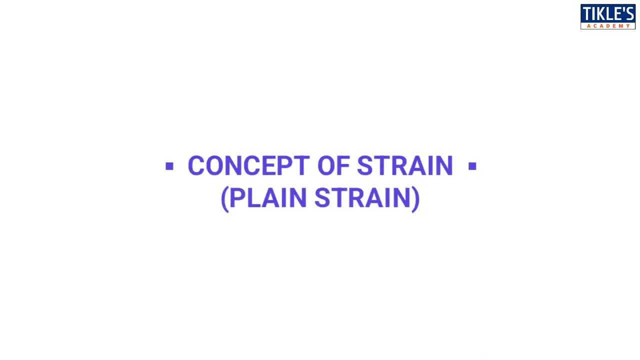 the power 3.. M stands for mega, that is, 10 to the power 6, and G stands for giga, that is 10 to the power 9.. So that's all about the concept of stress. Now let us see the concept of strength, that is: 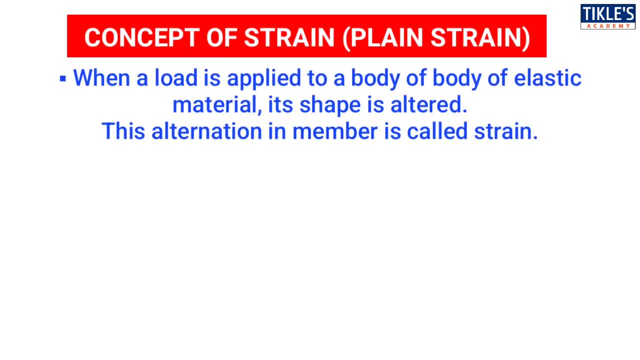 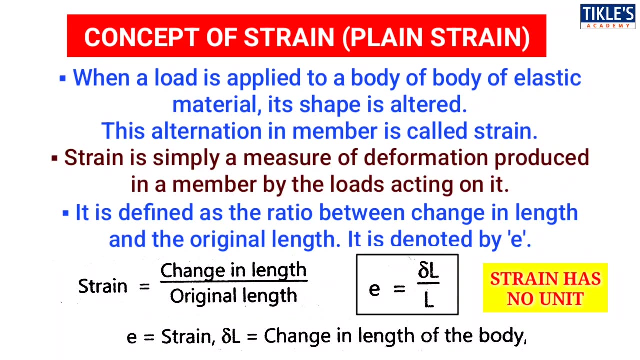 plane strength. When a load is applied to a body of elastic material, its shape is altered. This alternation in member is called strain. Strain is simply a measure of deformation produced in a member by the loads acting on it. It is defined as the ratio between the change in length and the 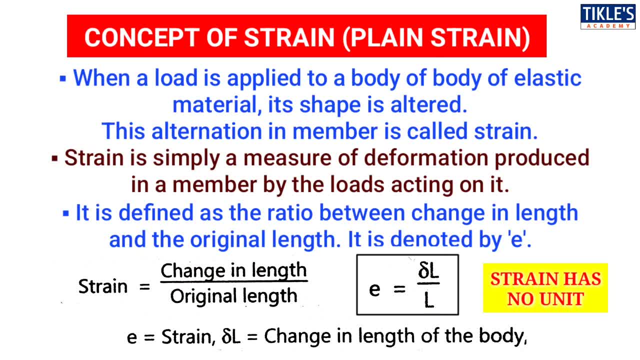 original length It is denoted by small e and, given by strain, equals to change in length divided by original length. So therefore, small e equals to del L divided by L, where small e is the strain del L divided by L. So this is the difference between the change in length and the original. 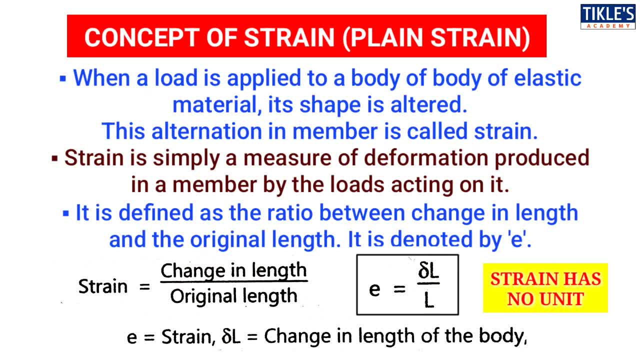 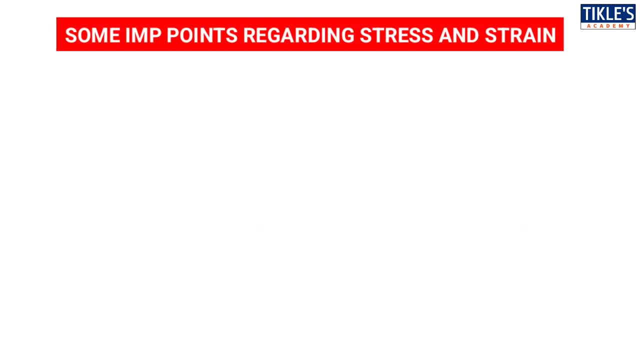 length Del. L is the change in length of the body and L is the original length of the body. Now let us see the unit, Strain being the ratio of two similar quantities. hence strain has no unit. So that's all about the concept of strain. Now let us see some important points regarding stress and 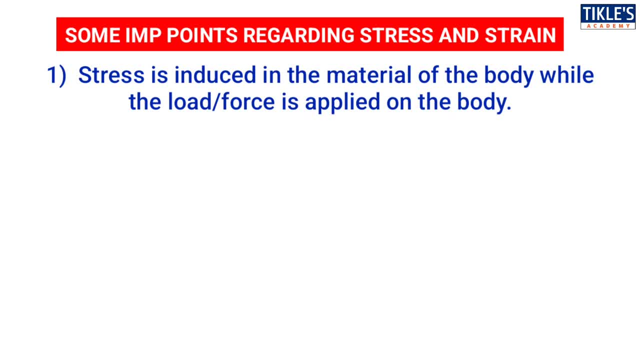 strain. So point number one: stress is induced in the material of the body while the load or force is applied on the body. Second point: the stress is induced in the material of the body while the load or force is applied on the body. So here in particular we are saying that strain gesture. 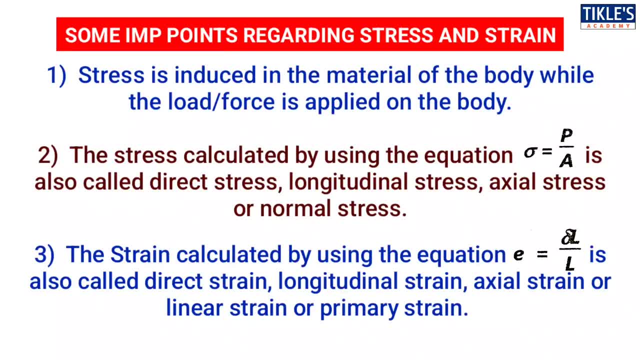 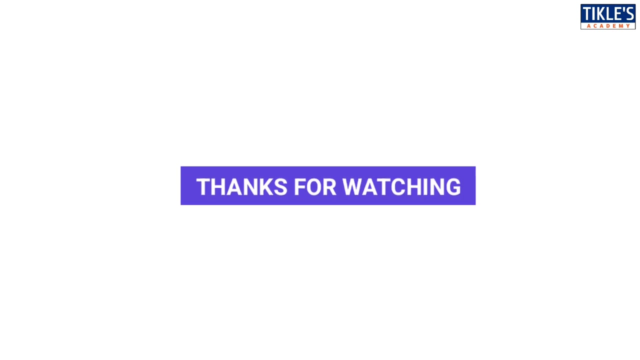 gives lift of the weight raising regarding stress and strength. so that's all about today's topic. meet you in the next video with some new topic. thanks for watching.